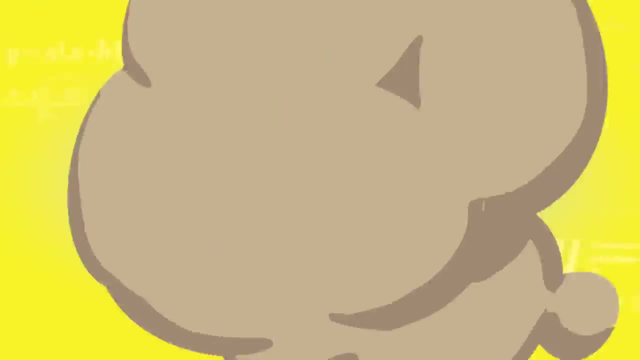 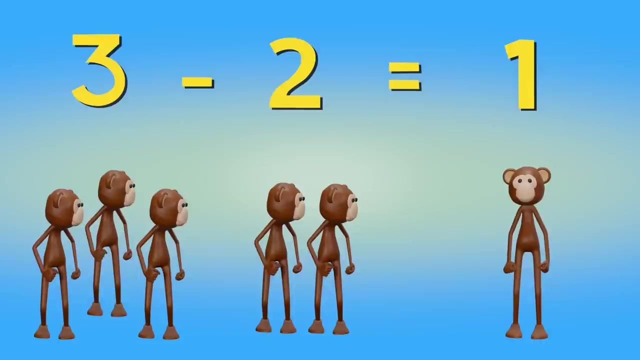 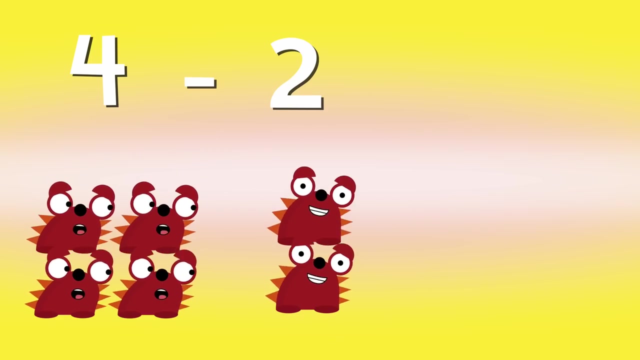 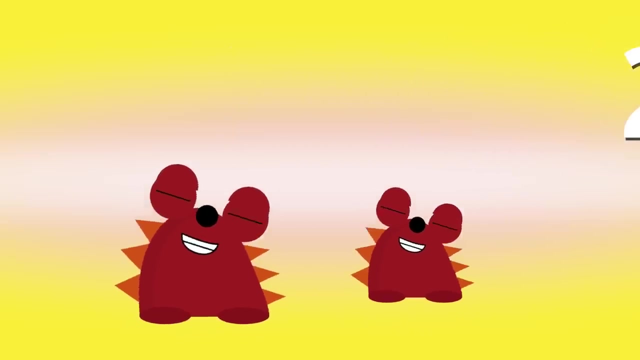 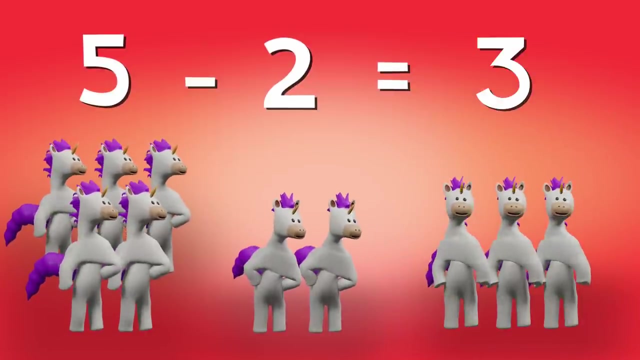 Magically mixing the numbers so I can do it all. Three Monkeys minus two Monkeys equals one monkey. Four Wigglers minus two Wigglers equals two Wigglers. Five Unicorns minus two Unicorns: Three Unicorns minus two Unicorns equals three Unicorns. 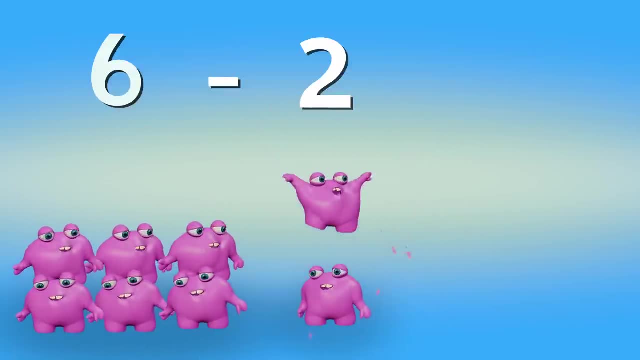 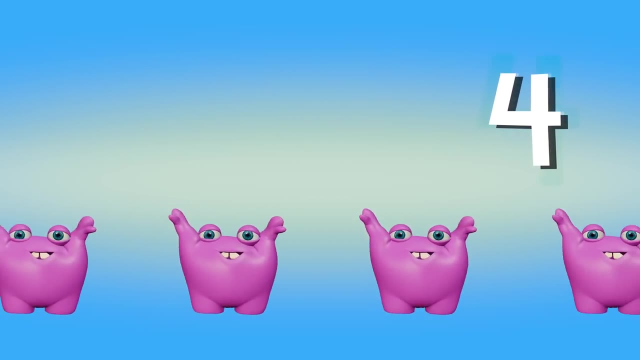 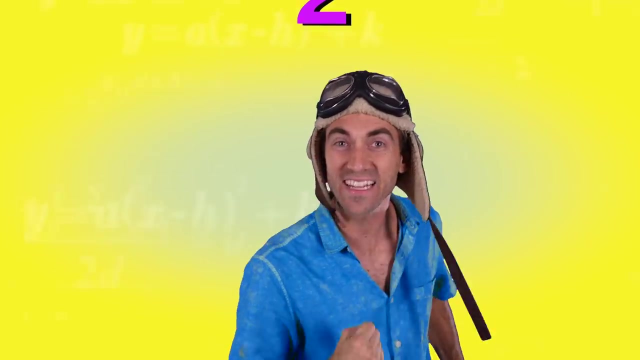 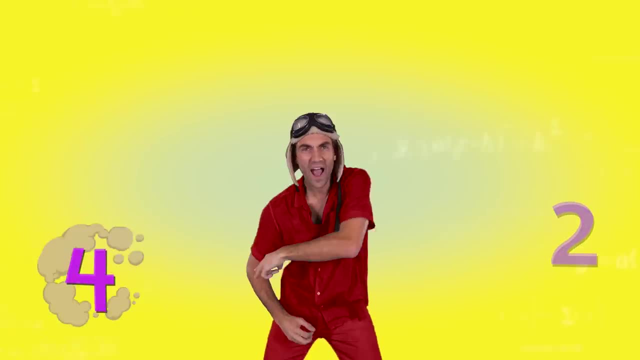 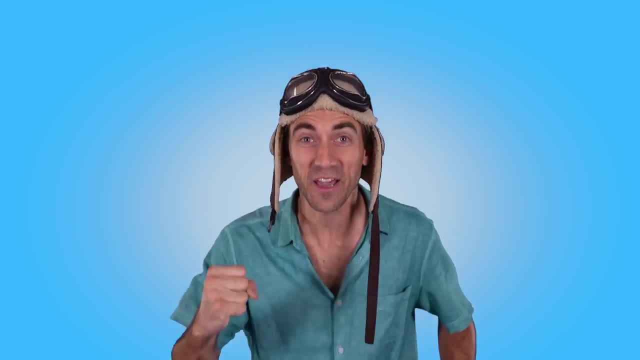 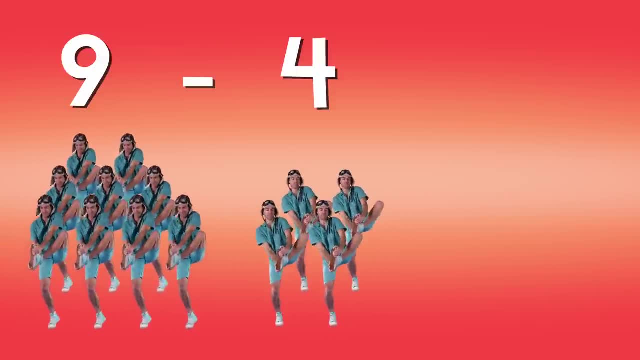 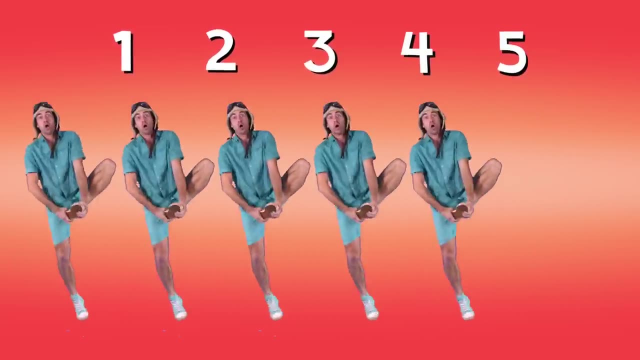 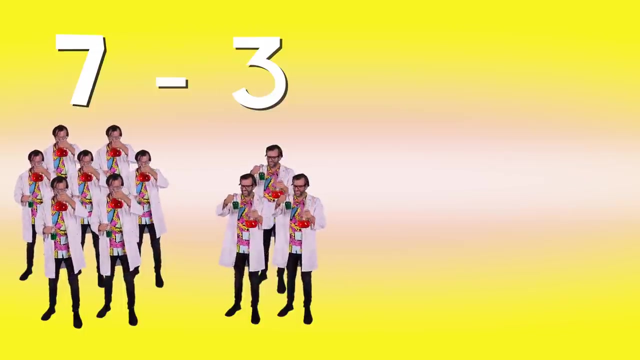 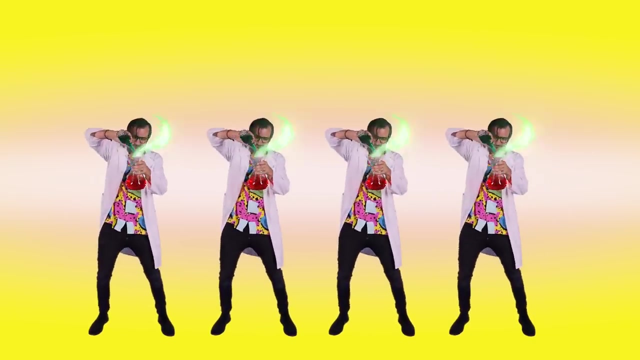 Minus four Dannys trying to get their shoes off Equals five Dannys trying to get their shoes off. Seven Papaps mixing chemicals Minus three Papaps mixing chemicals Equals four Papaps mixing chemicals. Eight Mini-Mangos pruning pineapples. 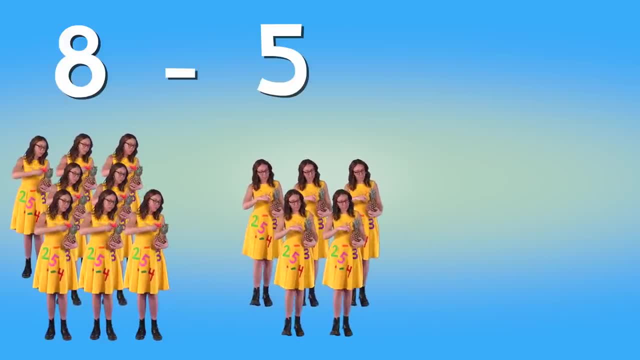 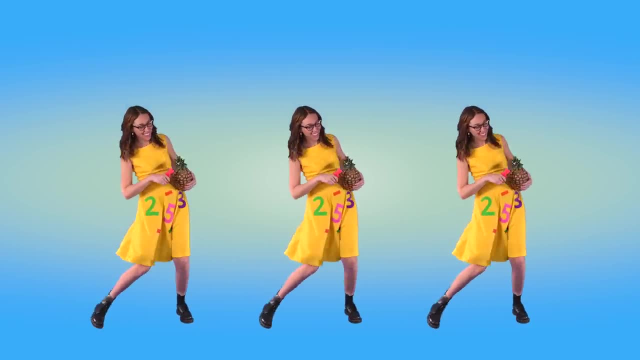 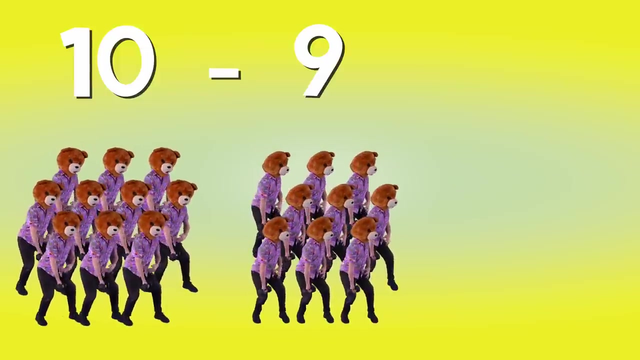 Minus five Mini-Mangos pruning pineapples Equals three Mini-Mangos pruning pineapples. Two Bearheads exercising Rrrr, Rrrr Minus nine Bearheads exercising Rrrr, Rrrr. 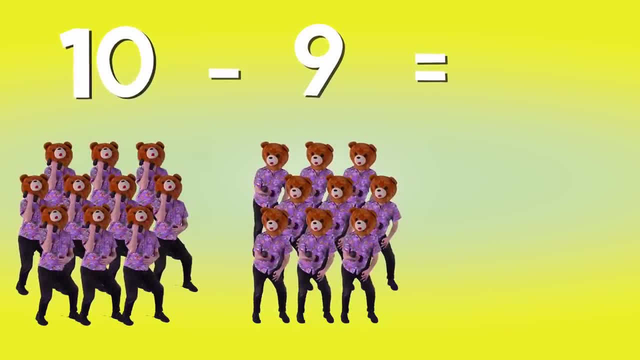 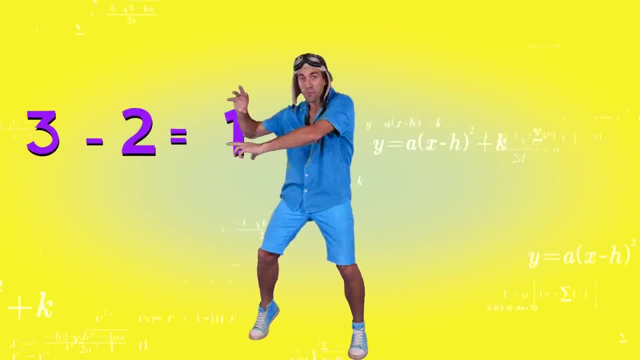 Equals. Can you get it? Rrrr, One Bearhead exercising Rrrr, Rrrr, Rrrr. I'm a math whiz. I'm a math whiz Magically mixing the numbers, so I can do it all.